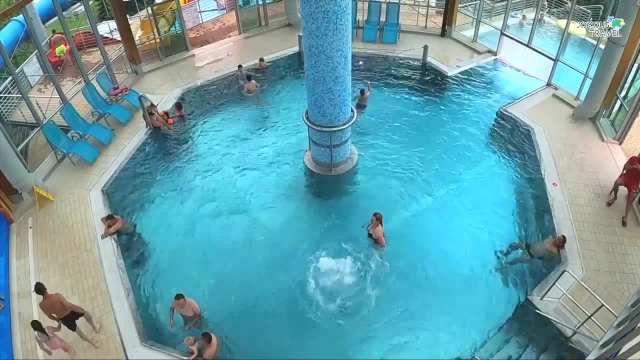 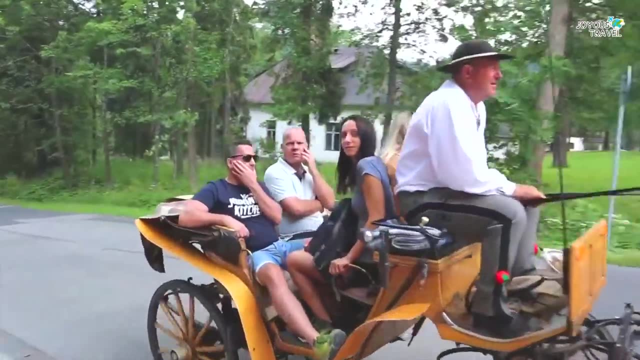 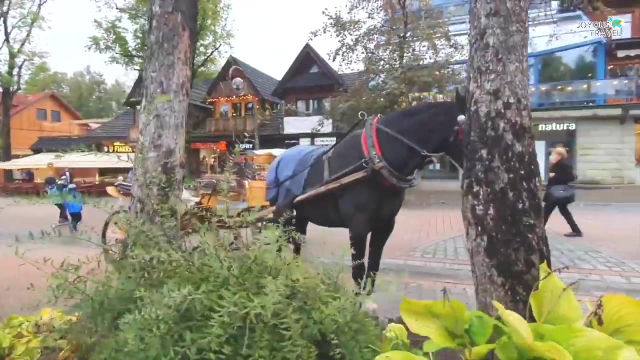 You will find everything from hot springs with a beautiful water park to various cultural activities. Zakopane is an exceptional city. Zakopane is an exceptionally varied city, wholly dedicated to tourism, with accommodation sites accessible to any traveler. Another attraction of this place is undoubtedly the Tarz Pod Gubawafka. 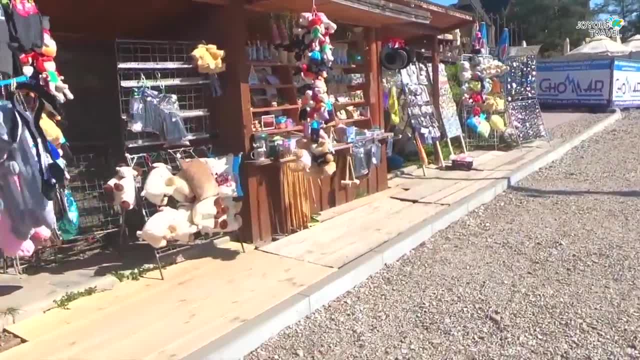 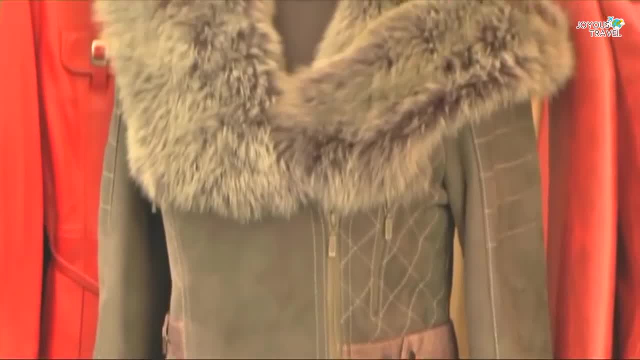 This highly diverse market offers beautiful souvenirs and handcrafts from the region, and vegetables and fresh food. Also, if you're looking for deals in coats and snowshoes, you can't miss this huge outdoor market Number 3. Tarnów. 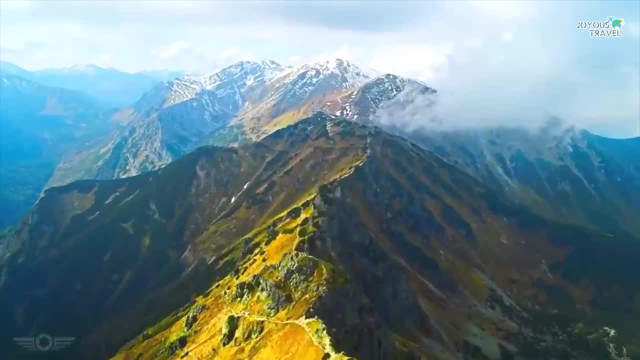 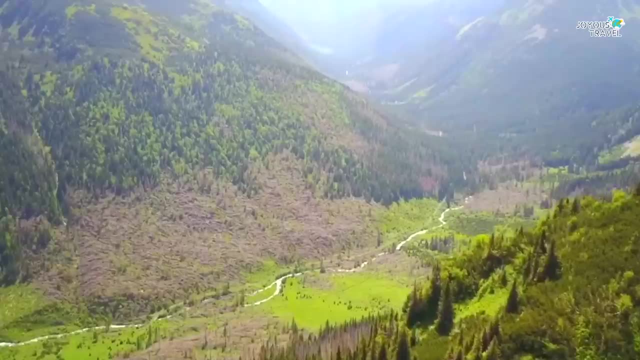 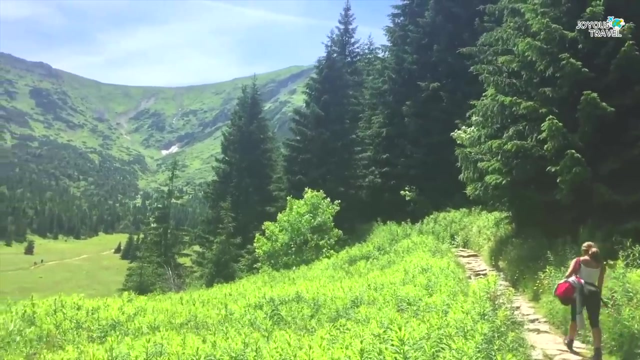 Tarnów National Park. Have you ever seen these beautiful landscapes on postcards? In this park, you will enjoy stunning views worthy of a panoramic photo. You will find incredible hiking trails, caves between snow-capped peaks and the famous Tatra mountains on the Polish side. 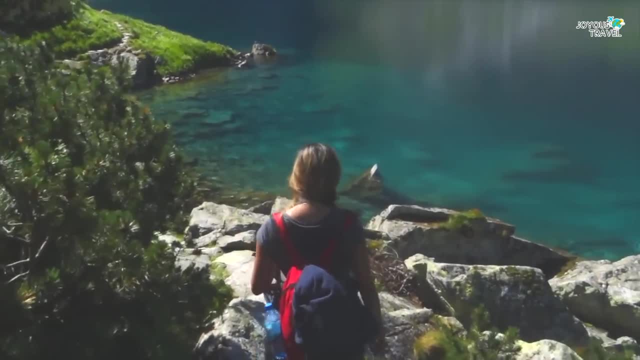 One of the main attractions of this place is the Morskie Oko lake. More than one hundred thousand people of all ages visit this lake throughout the year On average. the controllery is wearing a coral kiosk on theostral. 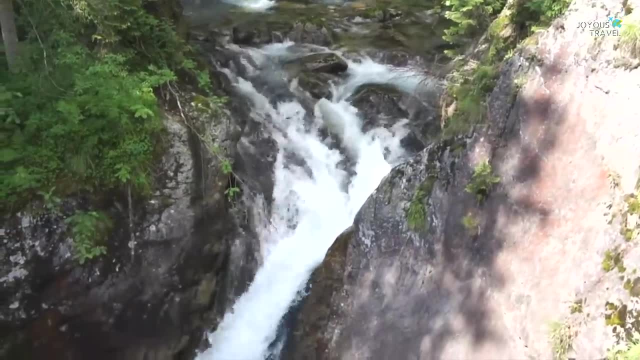 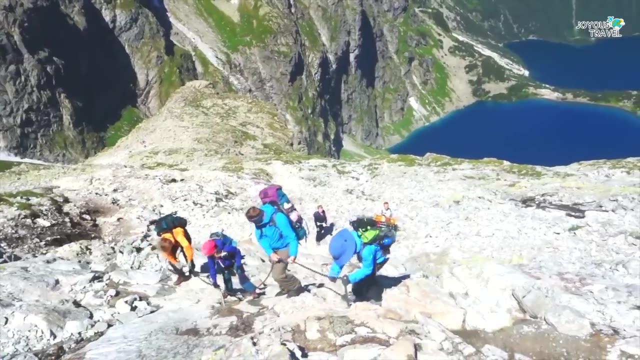 Number 3. Dink직bnica year. you can also visit the vodogushmote mitskevicha waterfalls. they're about an hour away from the lake. this park is the ideal destination for hiking enthusiasts or people who want to get. 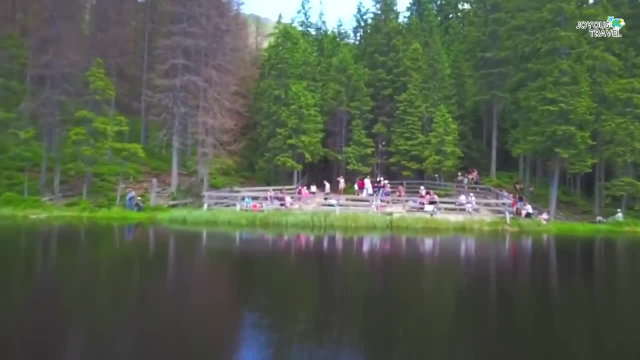 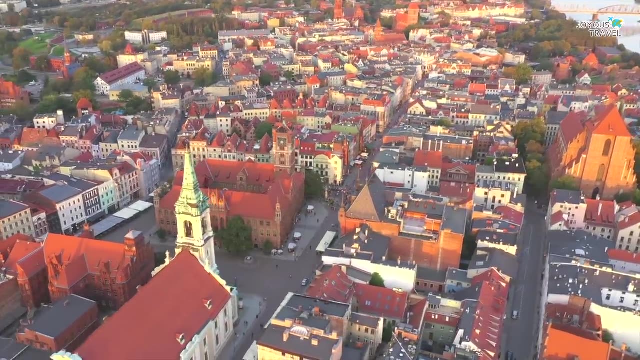 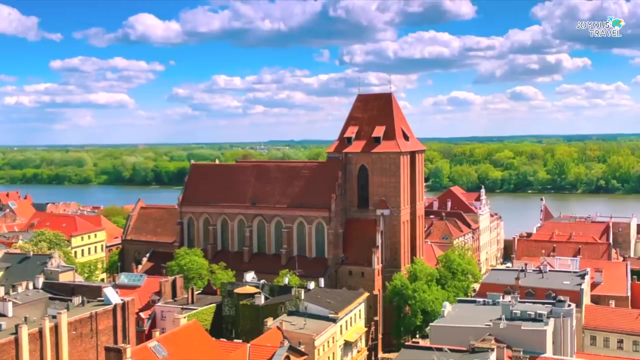 away from it all with outdoor activities. number four: toron. toron is one of the oldest cities in poland. this city is full of houses and buildings with gothic architecture, monuments that date back to the medieval age, thanks to the fact that it was not bombed or invaded during world war ii. 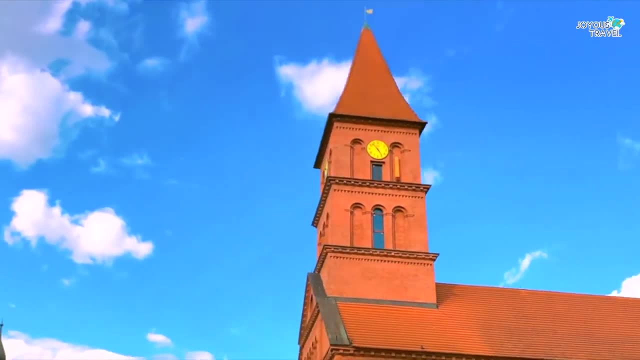 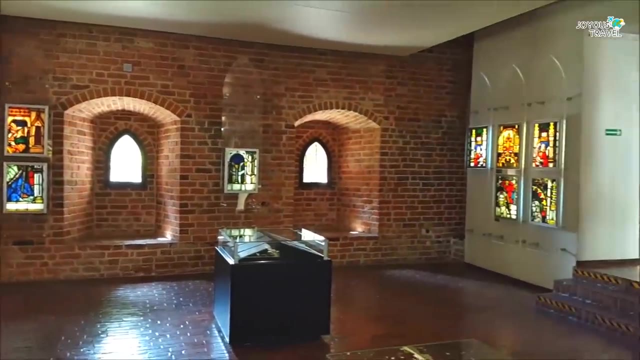 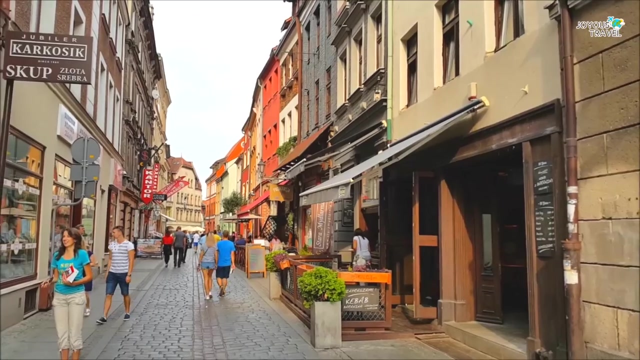 it still preserves excellent historical interest for tourists. you can visit the home of the most famous astronomer of the time, nicholas copernicus. it's now a museum and you'll learn a lot about his life's work and the contributions he's made to science. take a walk through the city and 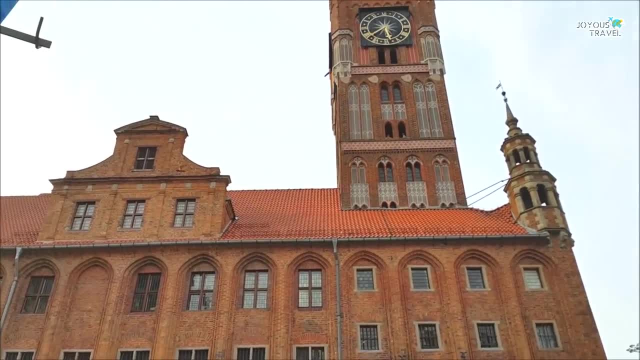 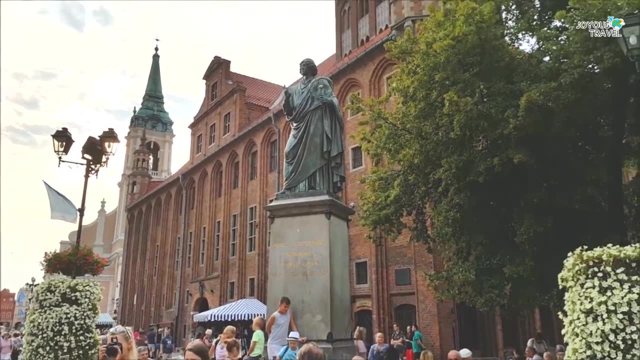 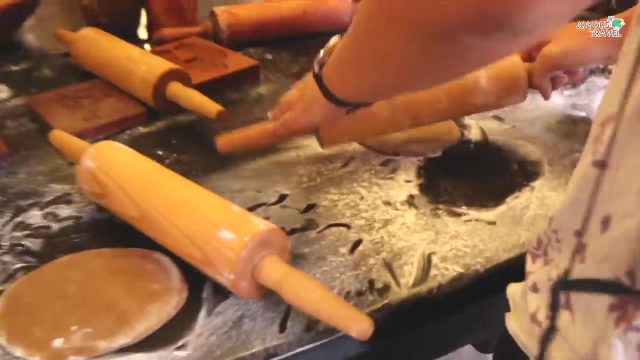 see the old town hall dating from the 13th century. nowadays it's a museum where you can know everything relevant to toron and its history. and if you're a baking enthusiast, we recommend you visit the city's gingerbread museum. have fun recreating all the steps to making. 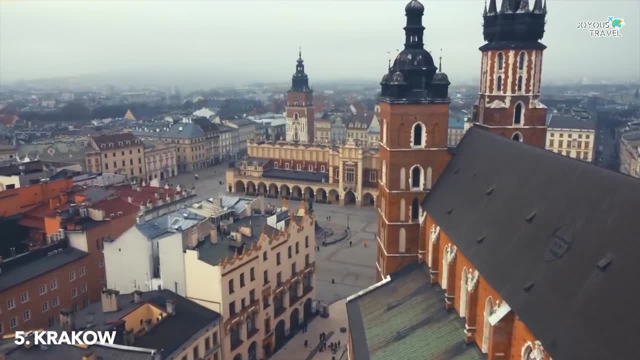 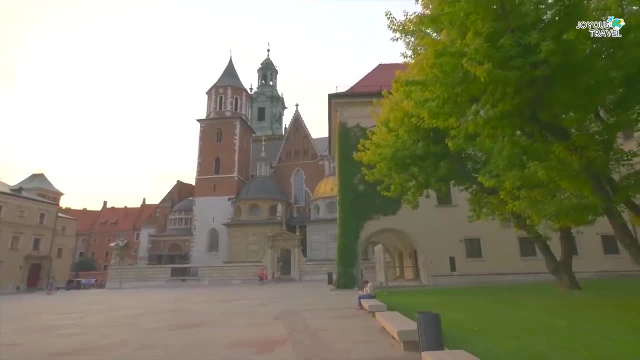 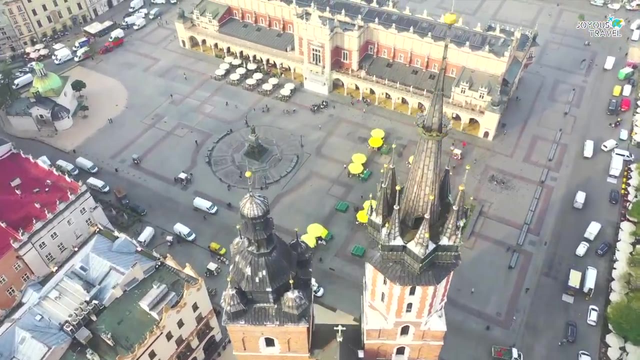 this delicacy. number five, krakow, or, in english, krakow. are you looking for a place where everyone knows your name? well, maybe not that intimate, but the tourist friendly city of krakow comes close. you can visit the market square, also known as renek guovni, the primary and social center of krakow. 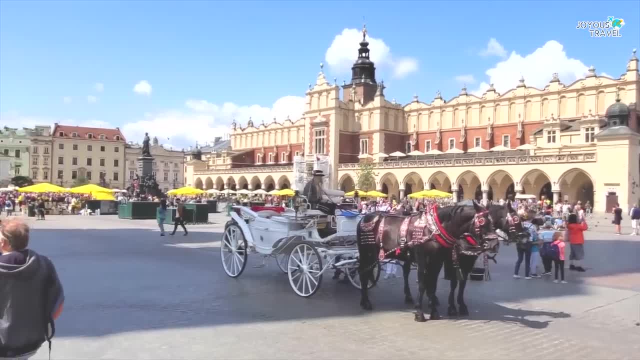 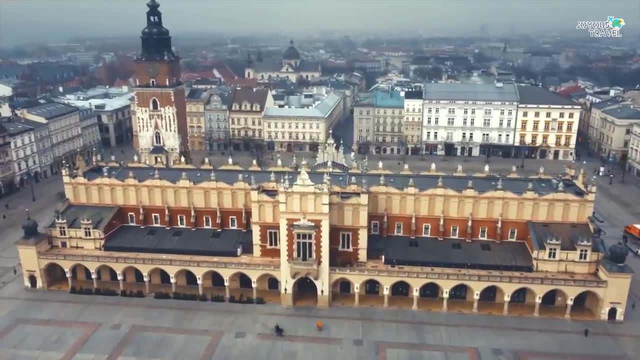 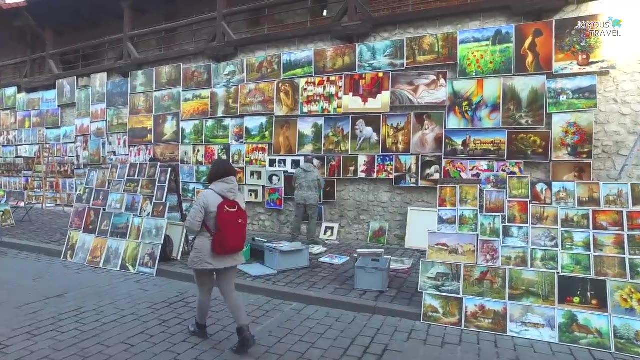 this square has been the protagonist of countless shows and cultural presentations, so if you're lucky, you'll enjoy one of them during your visit. pass by the cloth hall, known as the first covered shopping center in the world. another place of incredible beauty and architectural interest is the church of saint peter and saint paul. 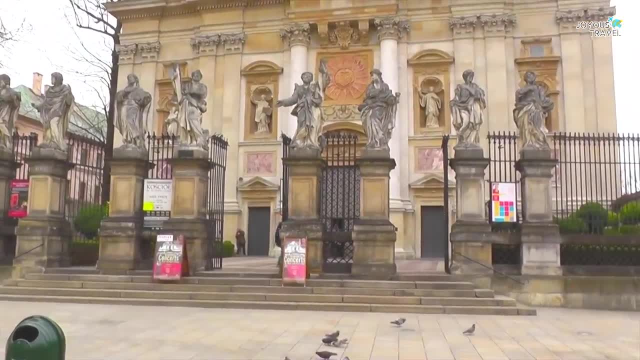 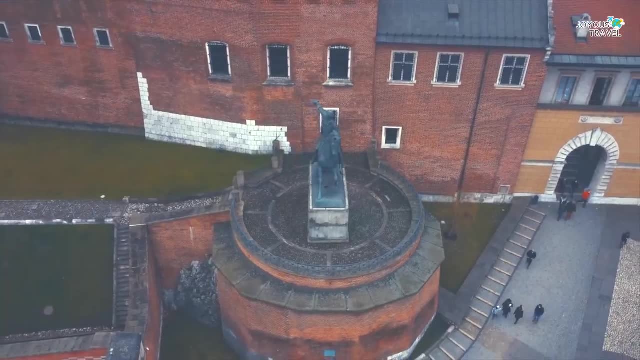 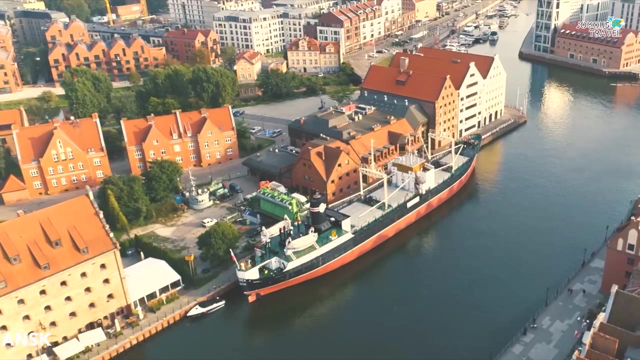 you'll see twelve statues representing the twelve apostles who stand as guardians of the church. this beautiful city stands out for its color, beautiful architecture and great artistic expressions. number six: gdansk. it's one of the most beautiful cities in the country. gdansk stands out for its history, architecture and excellent appearance. 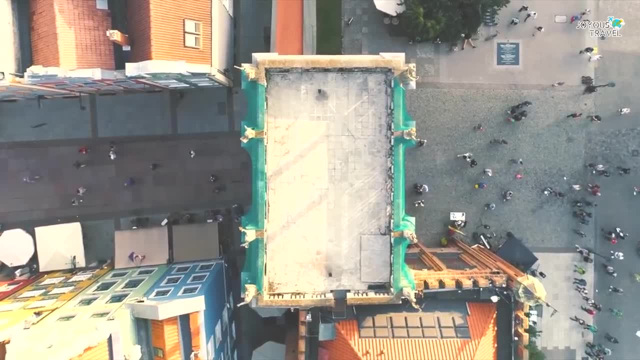 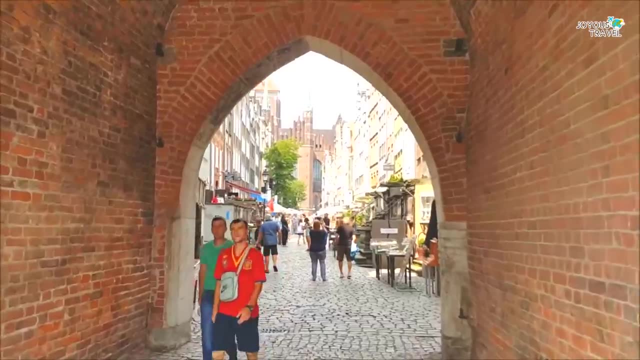 the site was a battlefield during world war ii, so it had to be rebuilt from the ground up. the city is a place of great beauty and beauty. and the city is a place of great beauty and beauty. you'll be able to get a hint of that dark time as you walk around the city. 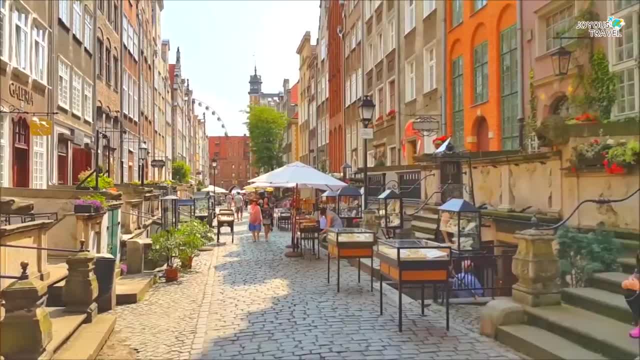 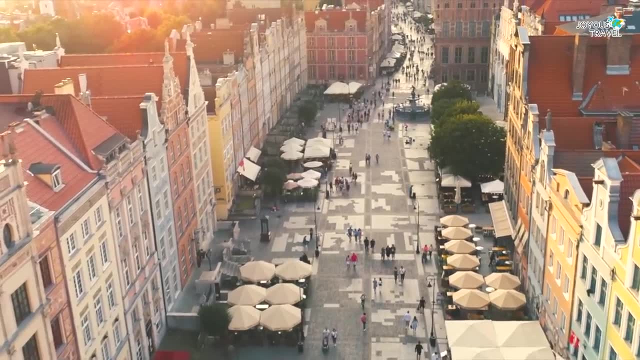 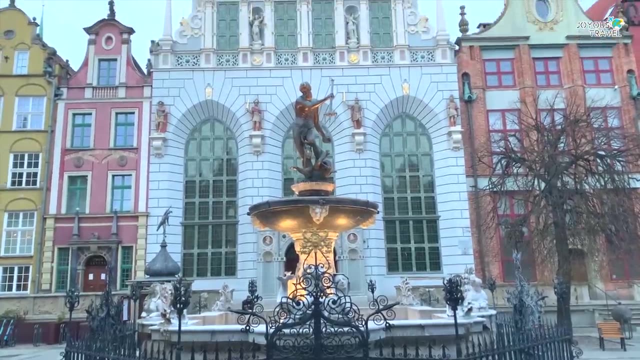 one of the mandatory stops you must take here is at amber street, known for being one of the most beautiful streets in the world. another notable area that you cannot miss is the royal route. it's a long street which once served as a path for ancient kings. with their entourage and 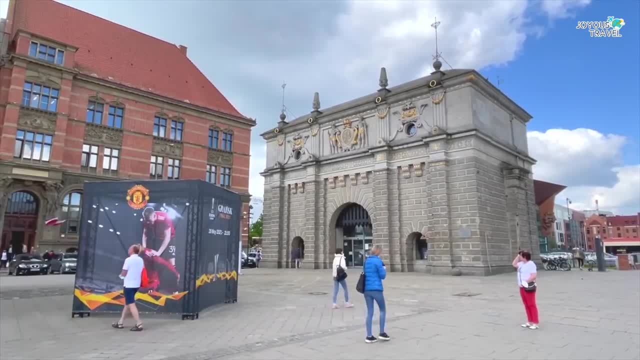 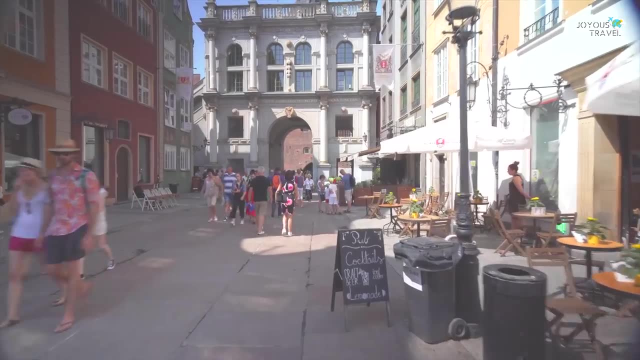 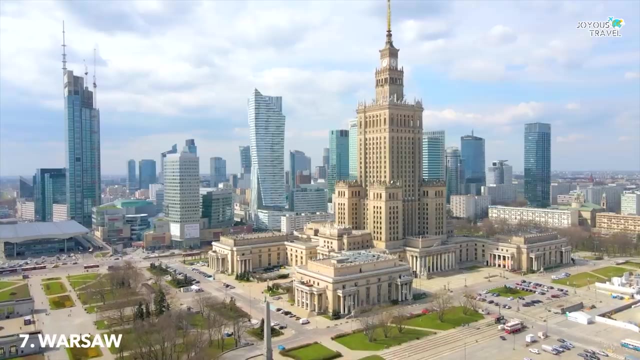 royal armies. your journey starts at the upland gate, passing through the city of gdansk and the passing through the main town hall, touring the houses of the nearby neighborhoods. this walk is a magnificent experience and shows you a bit of the history of gdansk. number seven: 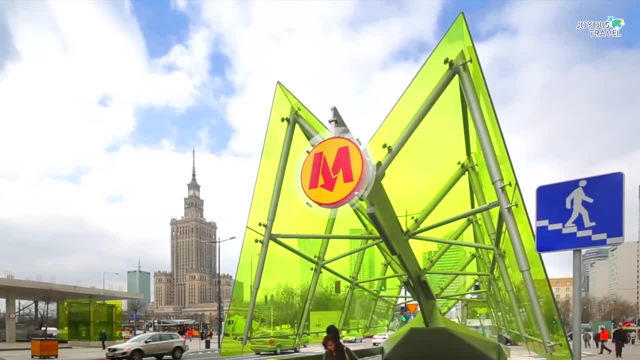 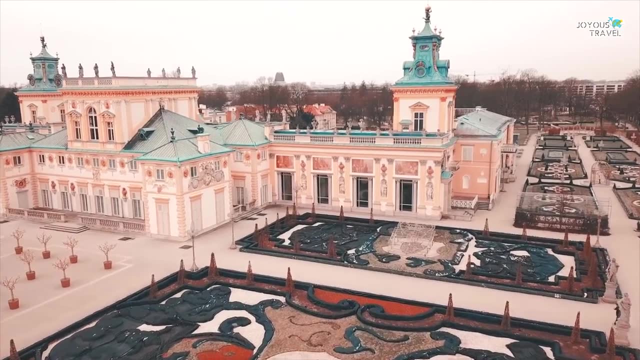 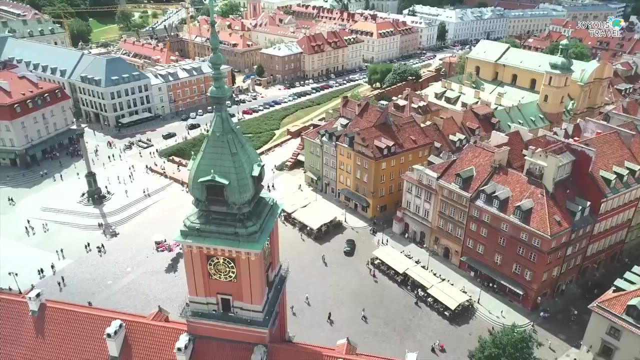 warsaw, or warsaw in english. for over 400 years, warsaw has been the capital of poland. the place was a victim of war and it does not forget its past while moving with passion towards the future. its most fundamental tourist attraction is the old town, declared a world heritage site by unesco. 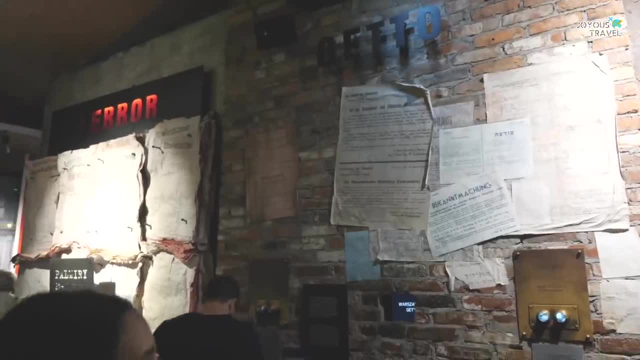 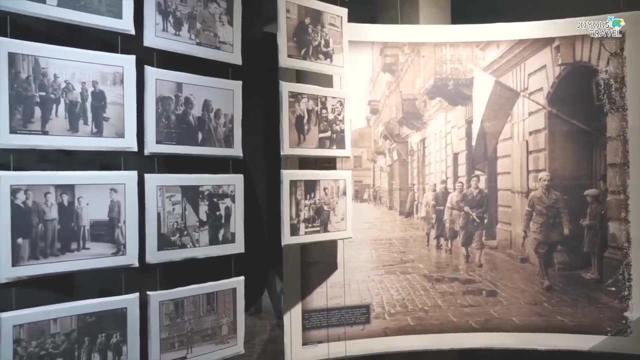 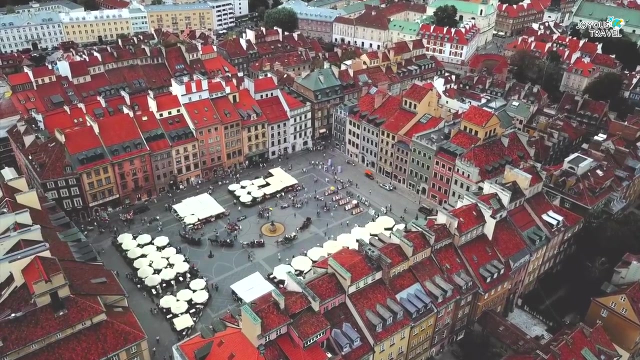 in the museum of the uprising you can learn the story of how this city stood up and fought against the advances of the nazi army, and how it resisted the onslaught of war. the warsaw old town market is one of the most beautiful squares in warsaw and was once the center of its public life. this square was built in the 13th century and 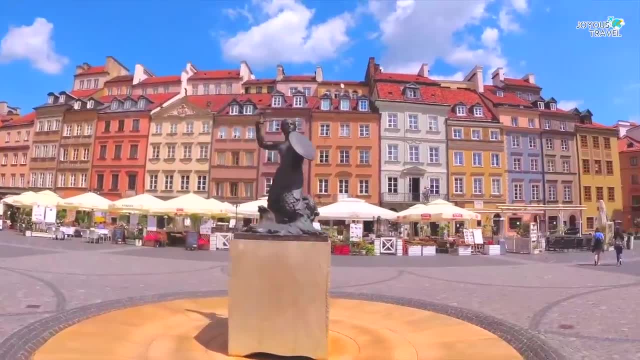 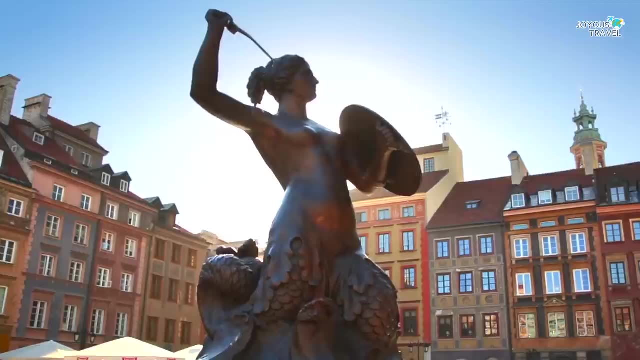 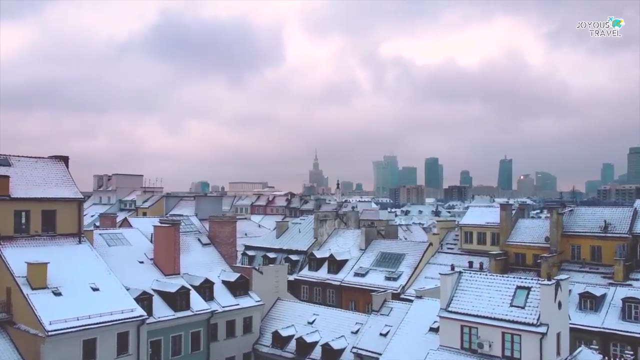 now. the constructions surrounded are from the 15th century. one of the city's main attractions and its most emblematic symbol is the little mermaid statue. a warrior mermaid is wearing a large shield and a sword, becoming the defender of the city when you travel here in the winter. 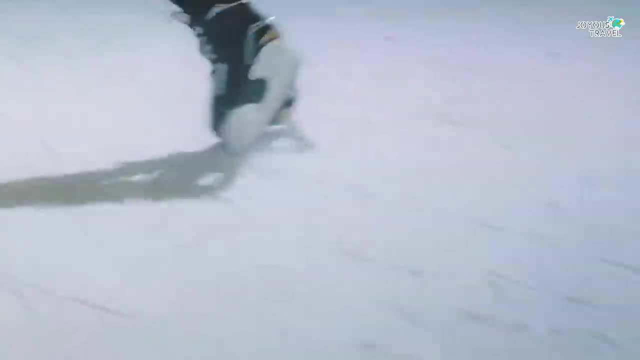 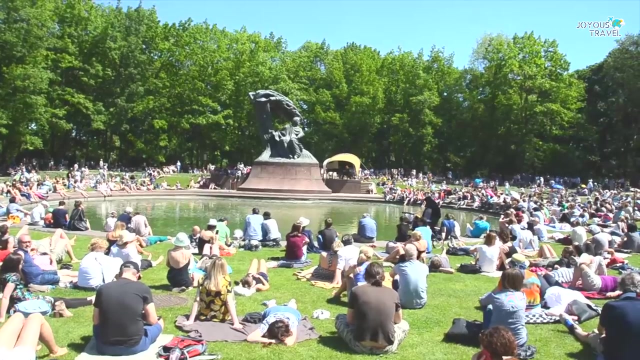 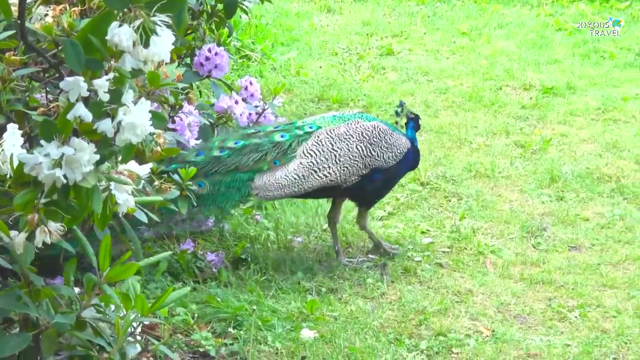 you must visit the ice rink surrounding the statue of the warrior mermaid. the wazhenki royal park is one of the most beautiful parks in warsaw. it hosts open-air classical music concerts and you'll love the beautiful gardens, royal belvedere and art nouveau. 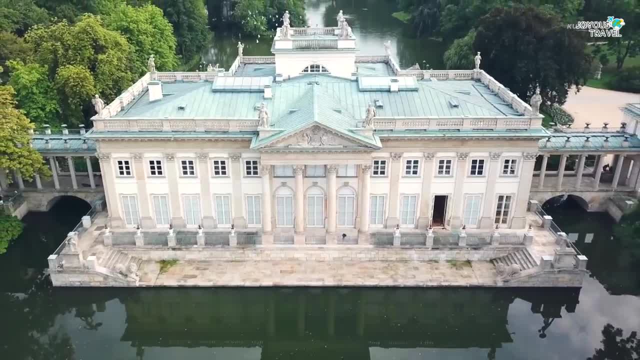 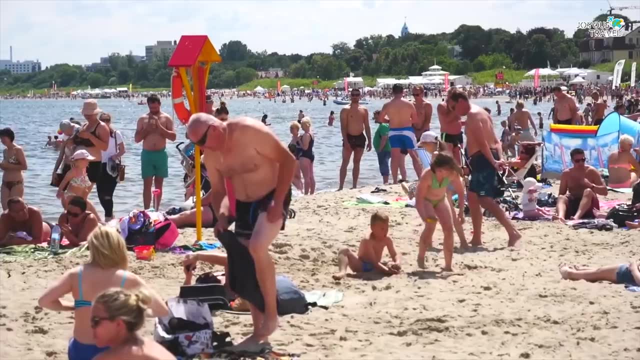 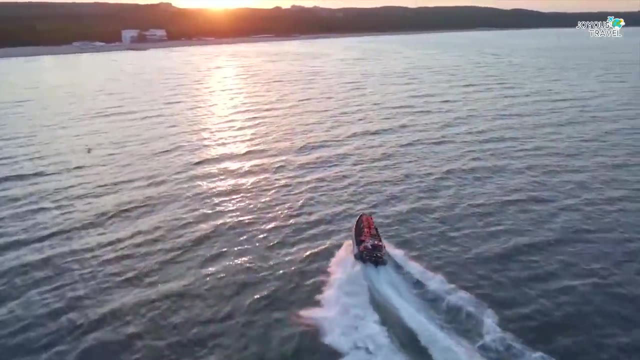 surrounding the large historical buildings inside the park. number eight: sopot. sopot is known as a seaside resort town with beautiful beaches, a large pier and moves between a quiet life and sporty highlights. the grand hotel is a huge building located at the foot of the beach. 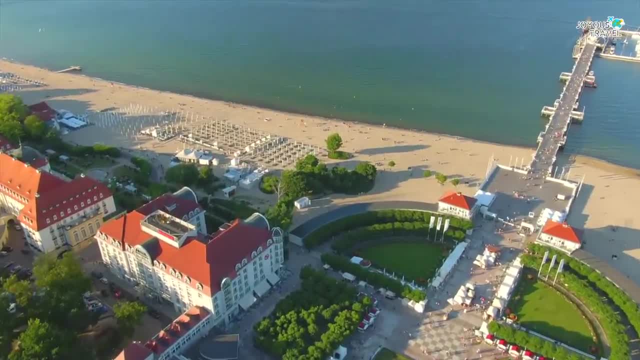 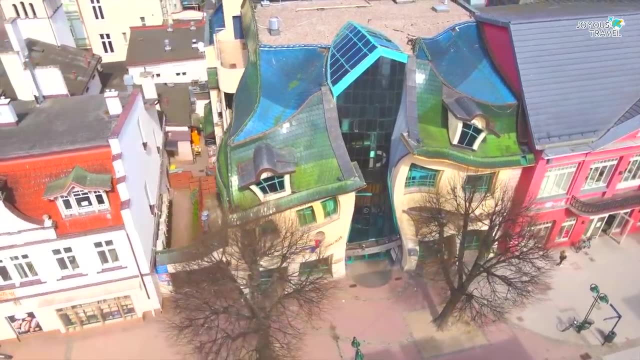 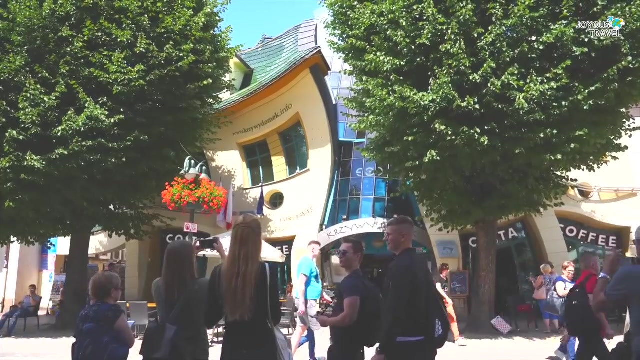 s王, of the oldest in the city. a great attraction for its particular architecture and its crazy design is the crooked house. it's a twisted shaped building that looks like something out of a cartoon designed by architects shotinsky and zaleski boatarov. monte casino street is a 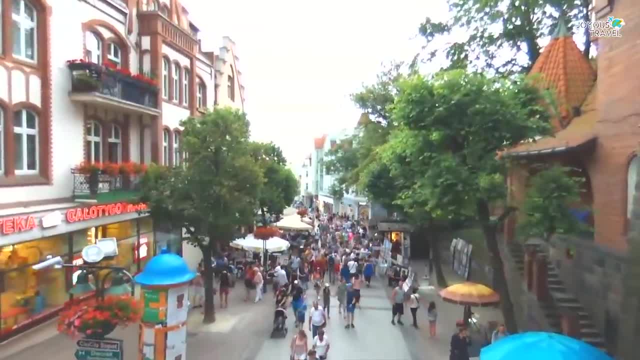 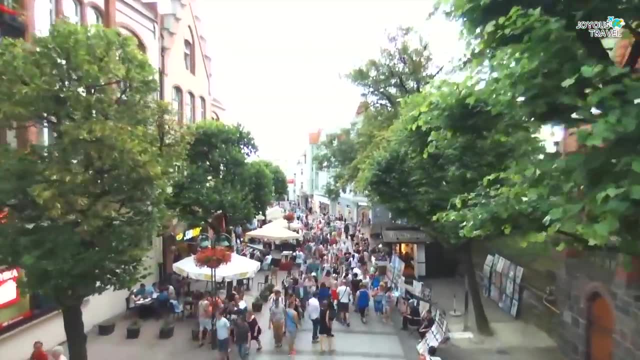 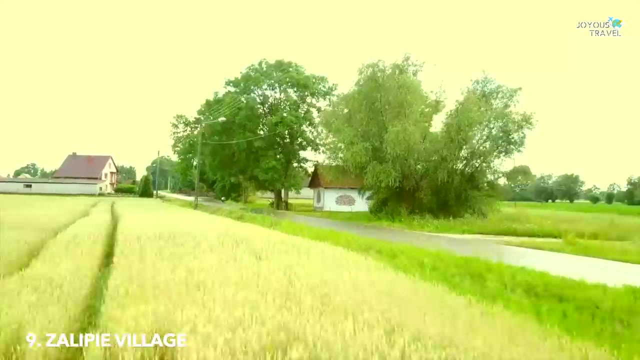 street primarily dedicated to tourists. you can walk without any difficulty through the souvenir stores, restaurants, cafes and clubs. you will find six unique propagations of local history and the and clubs located along this street. A quiet and comfortable walk that takes you directly to the pier of Sopot, Number 9. Zalipie Village. Are you looking for a colorful place to visit? 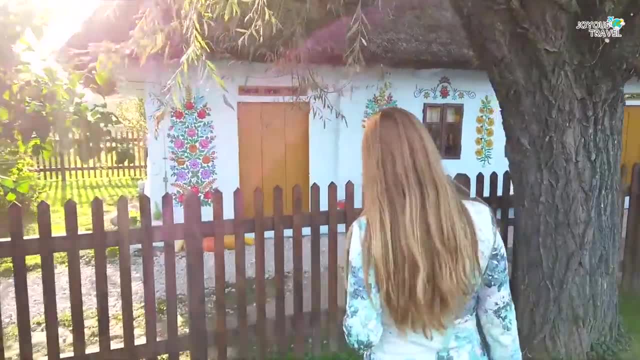 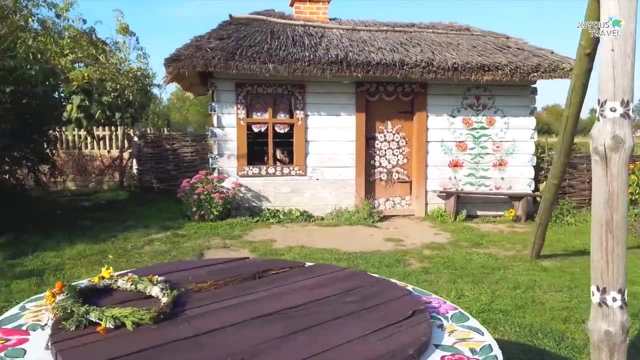 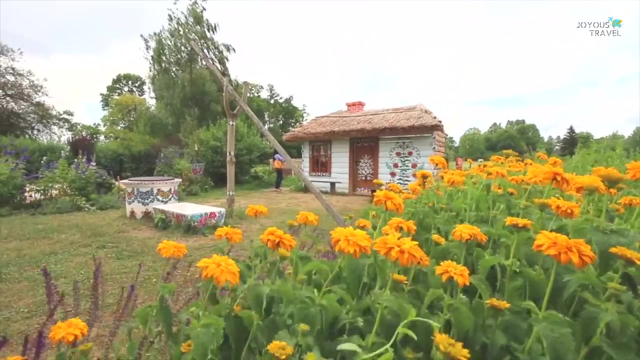 during your stay in Poland, Zalipie is the spot for you. Thanks to a local tradition that dates back more than 100 years, you can find colorful painted flowers all over any surface of the rural town. During your stay, you may run into some locals, Some of them open the door of their homes. 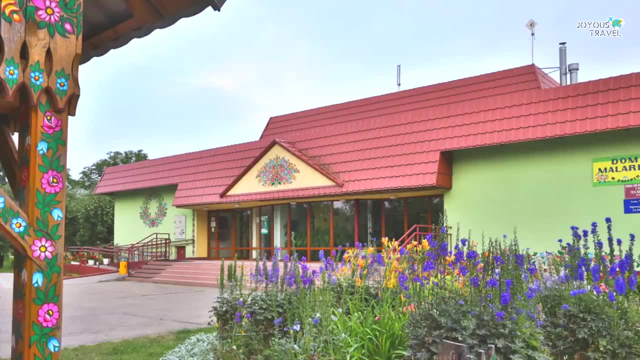 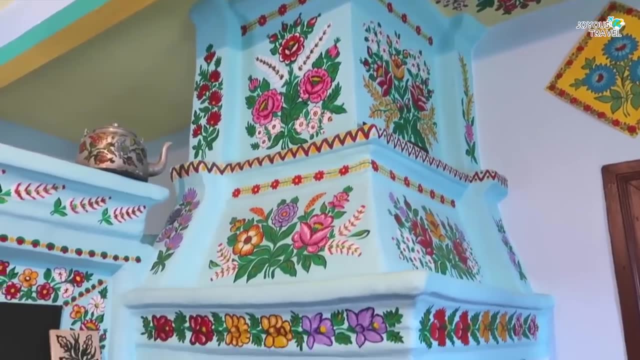 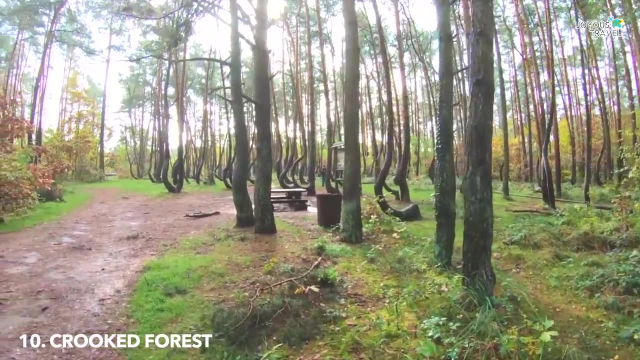 to tourists for photographs. Take a tour of the Dom Malarek Museum, or also known as the painter's house. There you can learn about local traditions and art through a variety of paintings and workshops. Number 10. The Crooked Forest. It's a forest of more than 400 pine trees with something. 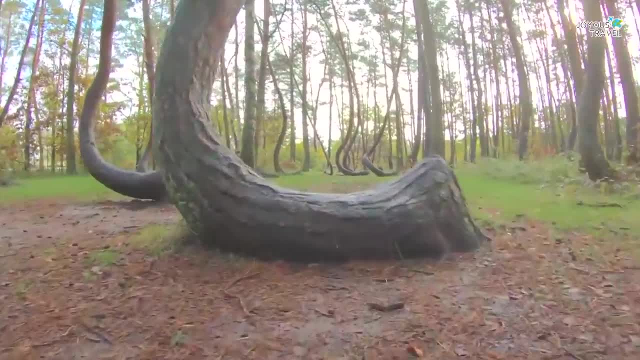 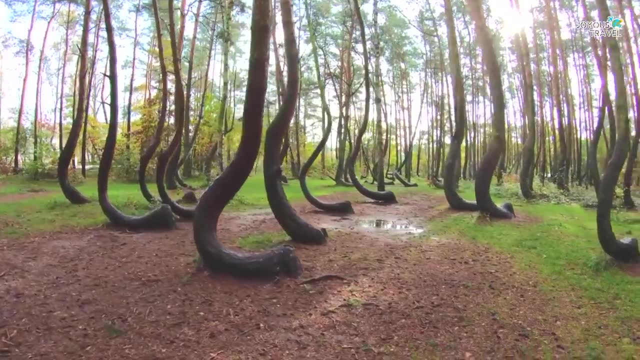 quite picturesque. Zalipie is a beautiful place to visit. It's a place where you can see the nature of the forest. The trees are peculiar and their shapes are bent as if they were the handle of a teapot. That's why it has become a unique attraction of the Polish territory. You can find 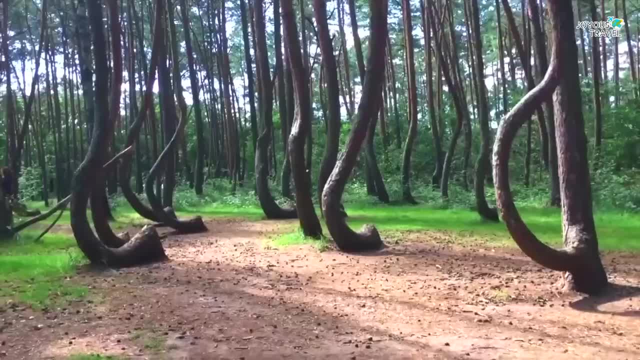 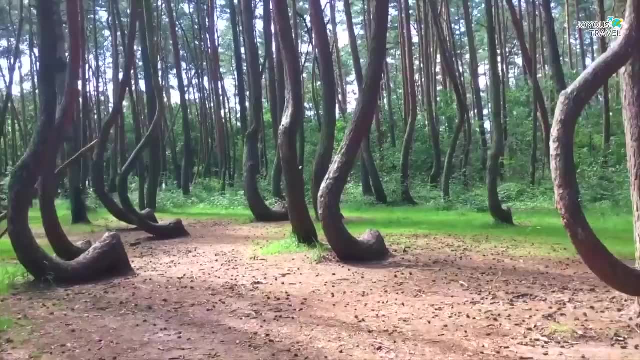 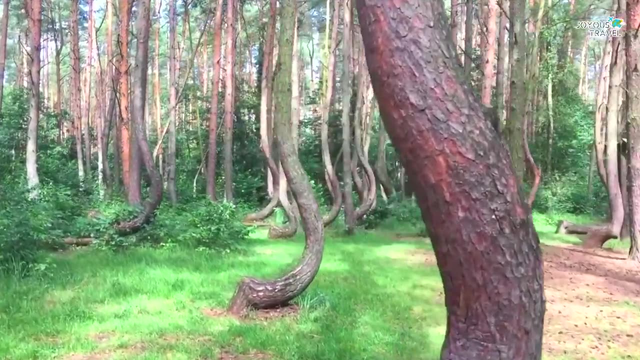 it on the outskirts of Nowy Czernowo village, very close to Grafino. There are many theories of why the trees of this forest grow this way. Some believe that it's something supernatural. Others explain that old farmers, in the middle of the growth of these pines, modified their forms to 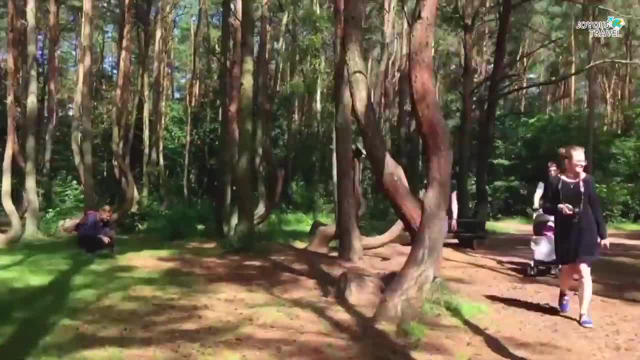 be used later in the manufacturing of the forest Number 11.. Zalipie: Are you looking for a beautiful place to visit? Downy Czernowo here makes its way Today. the mystery remains unsolved, which attracts the attention of tourists who visit this area. This beautiful country has. 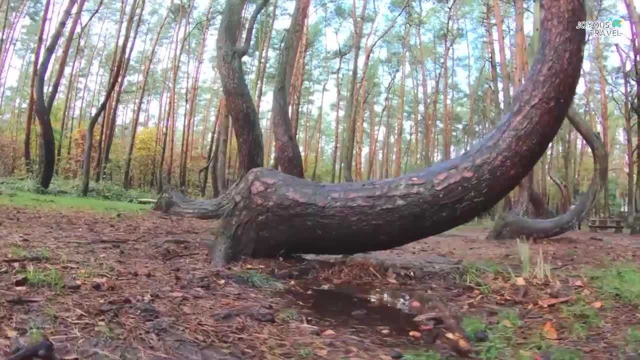 been through a lot – but despite it all, The incredible impetus of its citizens has kept it standing. Enjoy its delicious cuisine, which will make your taste buds explode. Let yourself be carried away by the great history of this fighting country. Discover Its charming. 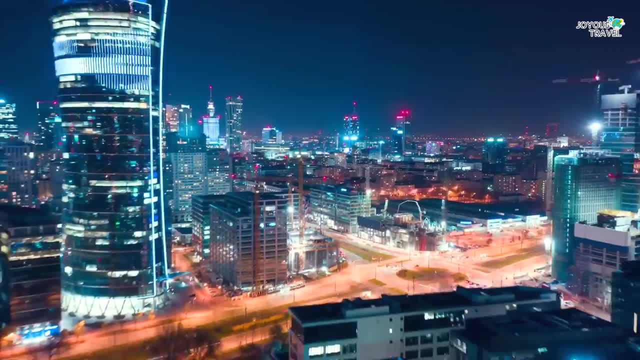 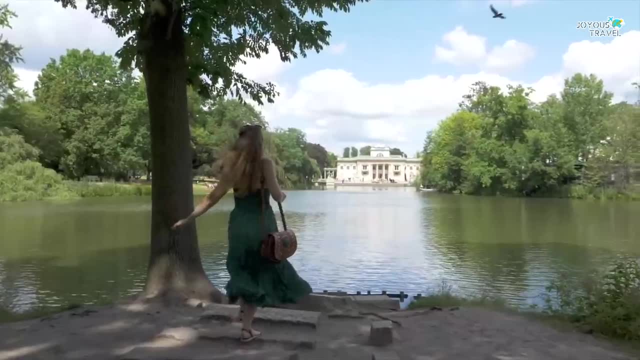 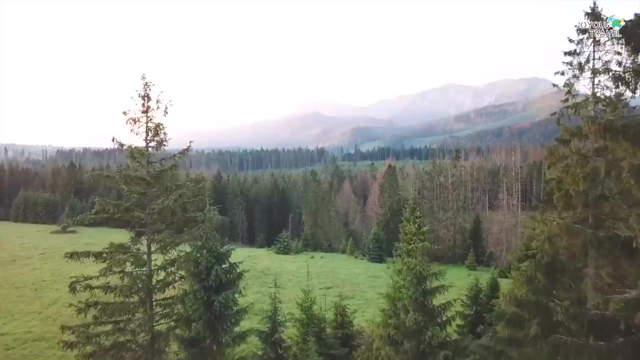 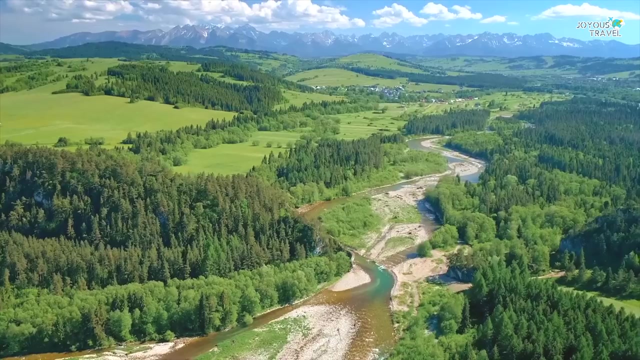 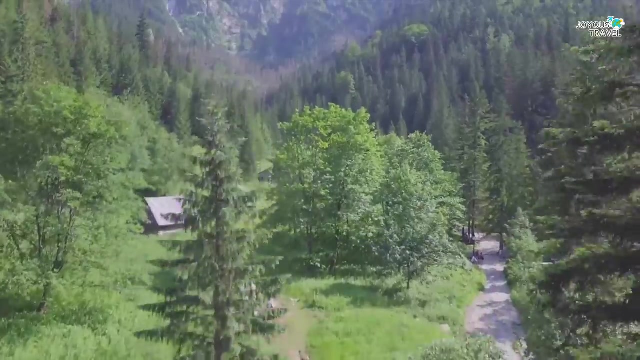 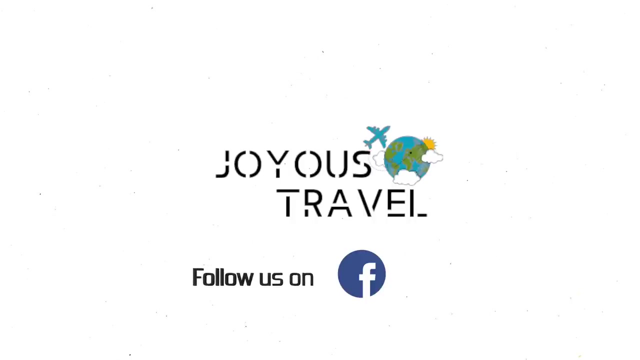 villages, main cities and, very well, Beregovany, mountainous areas and even beautiful beaches. so pack your bags and experience the phoenix of europe, poland. if you enjoyed this video, give it a like and click subscribe. thanks for watching so.